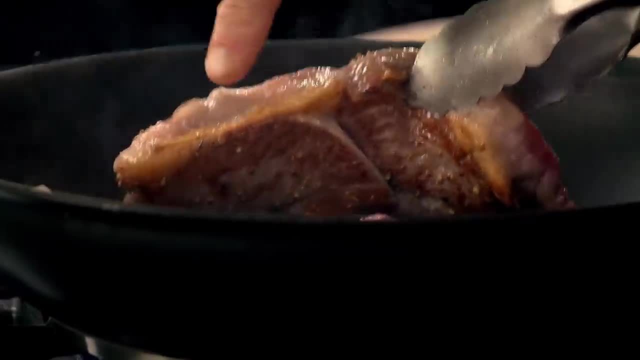 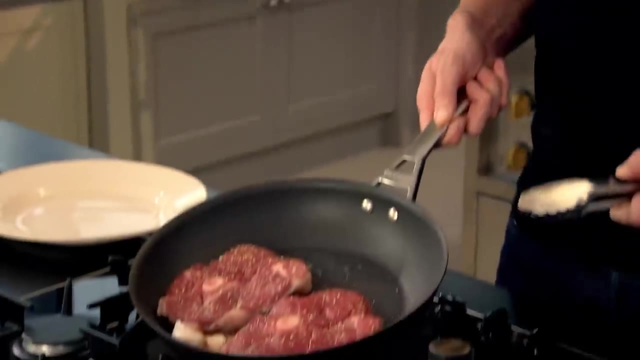 In tongs. lift up That bit of fat around the back that's at the top of the leg. Tilt the pan and let all that fat render. Rendering is a chef's term. That means melting the fat. It works brilliantly when you're cooking a ribeye as well. 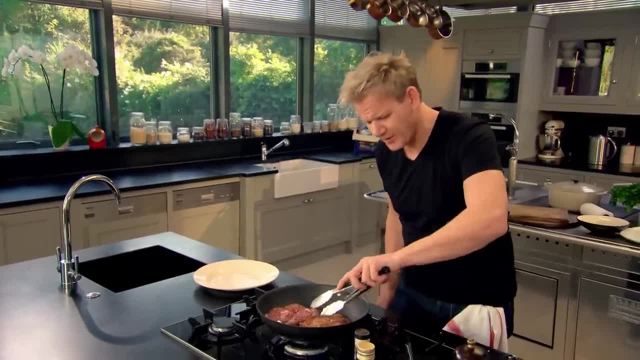 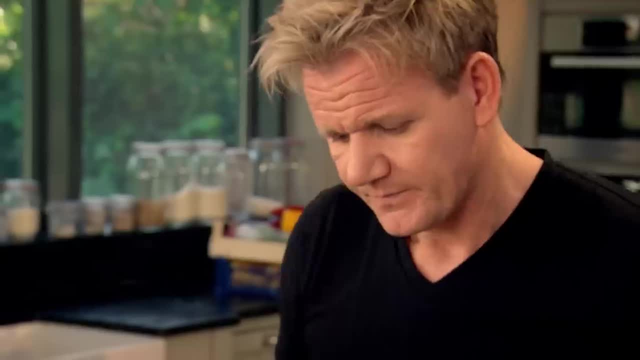 Cut it over. Look at that color there, Beautiful. Now it looks like an expensive cut and we've got that nice even sear all over As it's cooking. just tilt the pan and baste, And basting the lamb steak just means. 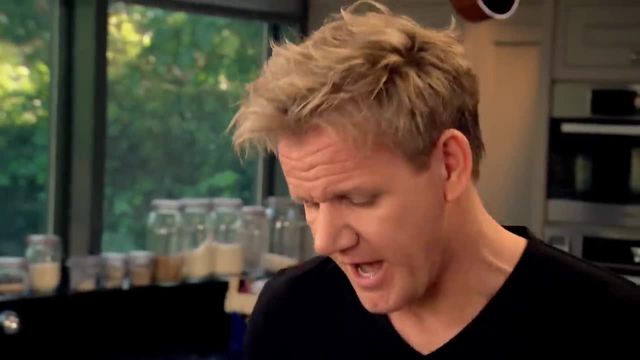 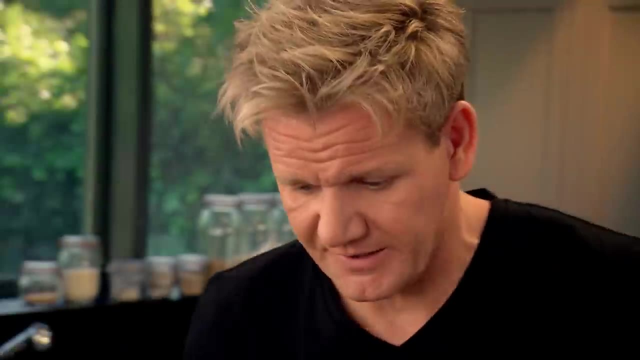 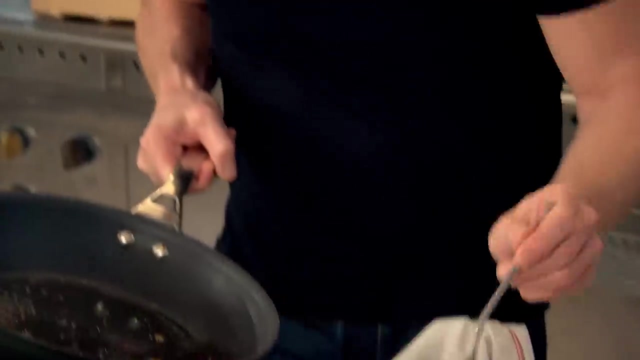 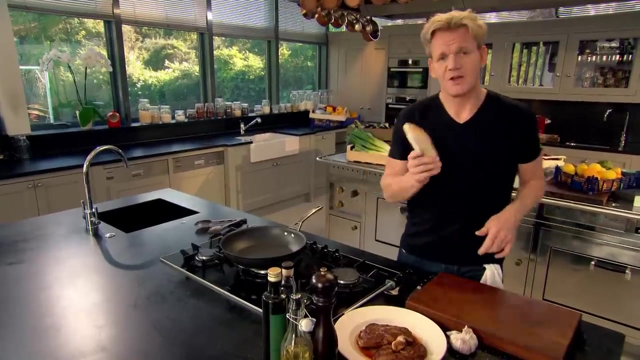 you're sort of adding all that nice scented garlic olive oil back into the lamb. Beautiful Now take the lamb out and let the lamb rest. Beautiful, Now For the perfect rustic crouton. So this bread's quite firm. 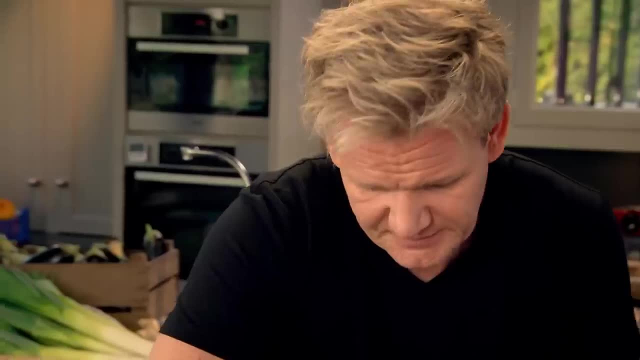 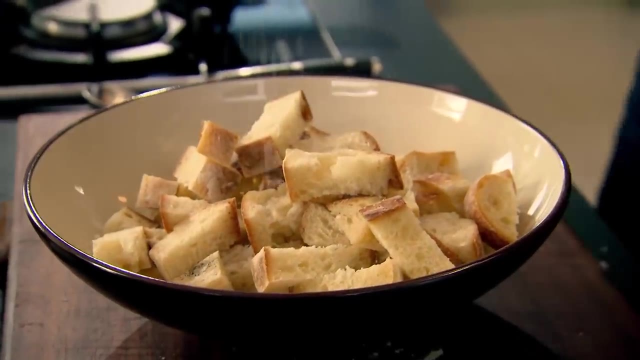 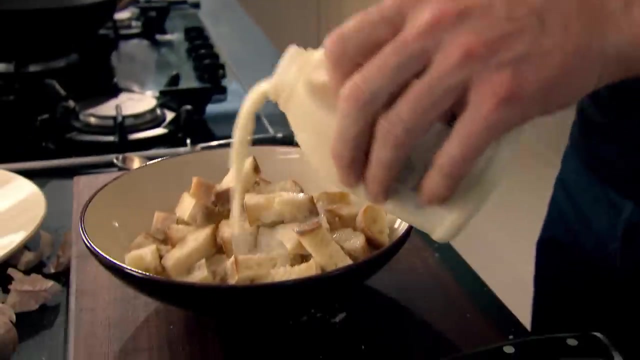 Couple of days old. Just slice it straight down the center, Dice it up, Put it into a bowl, Season it beautifully From there. I'm going to add some milk. Sounds strange adding milk to a crouton, but it just gives it that nice, rich, creamy texture. 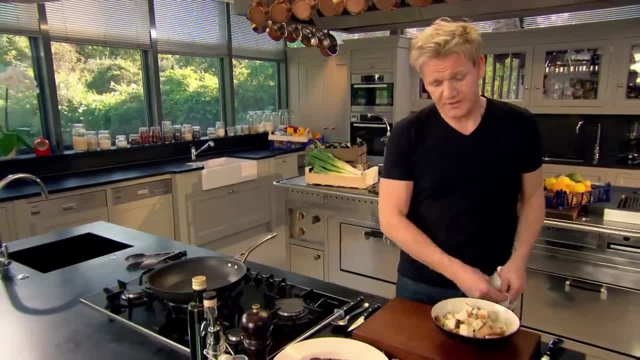 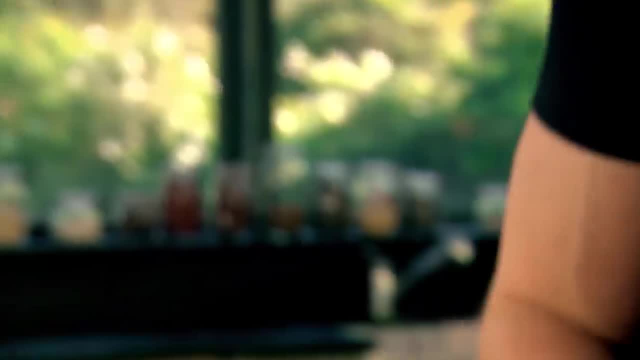 And just let that milk sort of absorb into the bread While that's soaking. I'm going to make the dressing Go back to that initial garlic that was in the pan- Look at that Beautiful Into the pestle and mortar Anchovies. 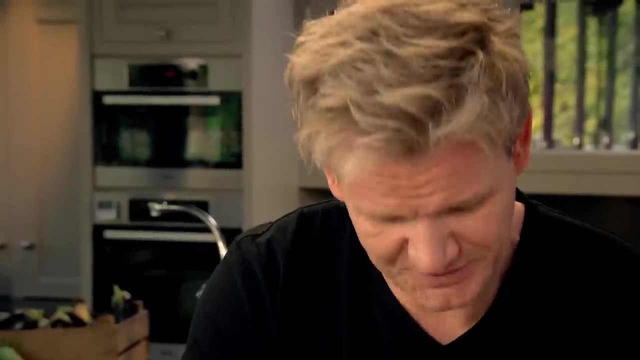 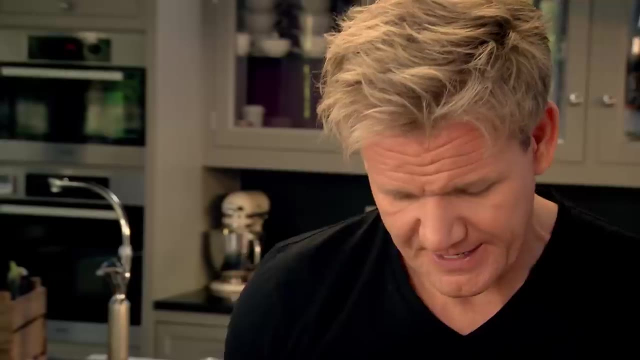 Anchovies go brilliantly well with lamb. I want that nice salty vinegary flavor And a bit of kick. Some capers, The little baby caps, Very sweet. Now just pound that to a nice paste That smells incredible. 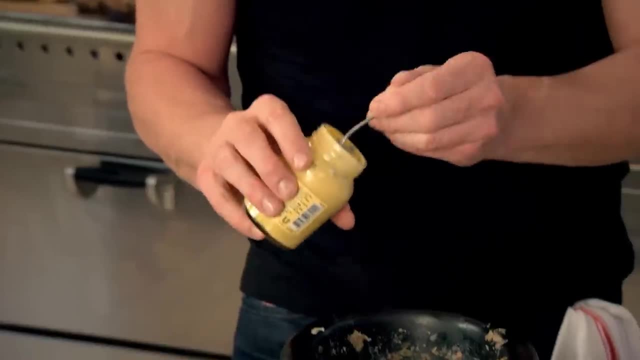 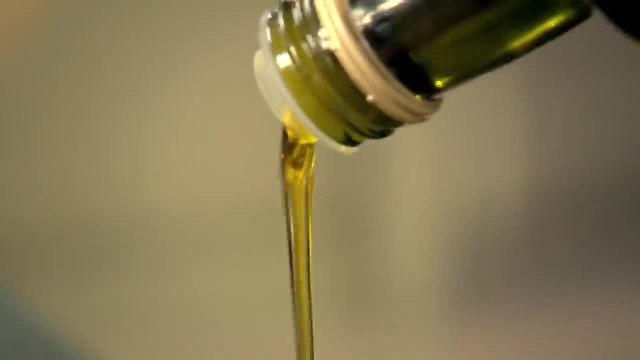 Next some Dijon mustard- A nice teaspoon and a half- in A little bit of red wine vinegar, Two tablespoons, And then our extra virgin olive oil. Now it's got that heat in there, Got that nice roasted garlic. 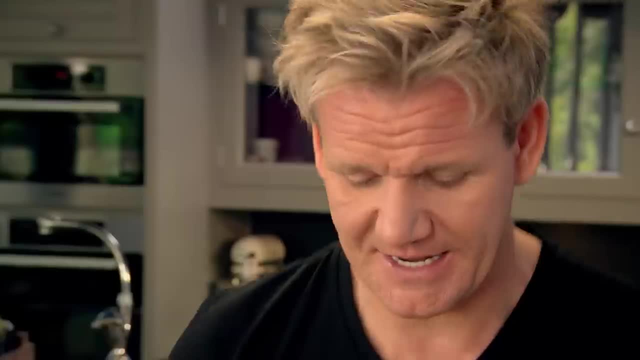 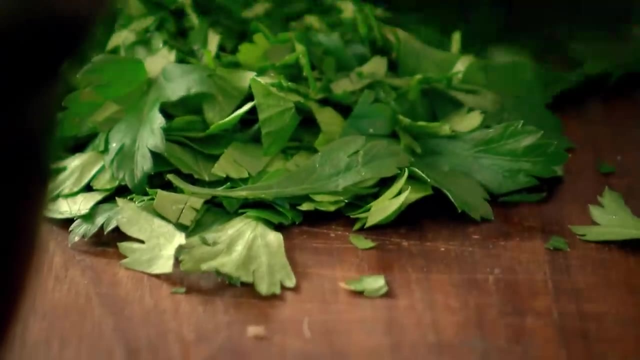 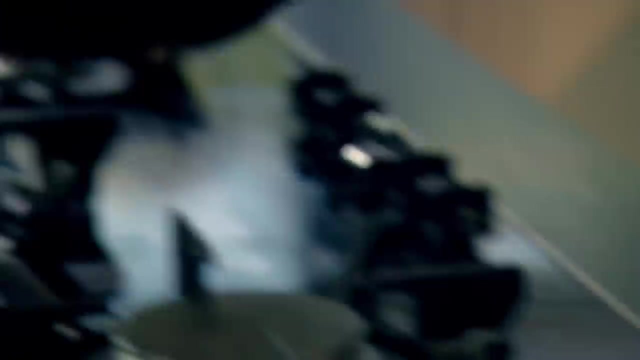 A real hearty, chunky vinaigrette that sort of seeps into that lamb Some fresh parsley. Crunch up the parsley Delicious flavor, Parsley in Nice. Now get your pan hot. for the croutons, Olive oil in the pan. 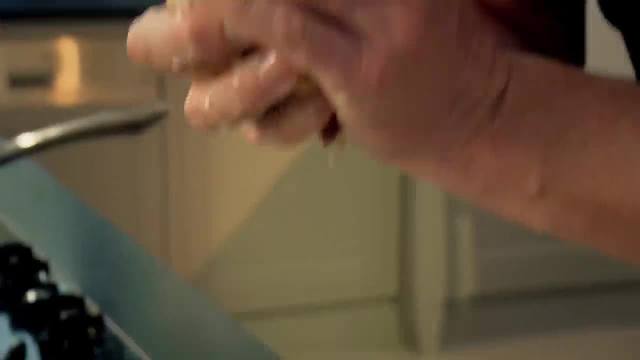 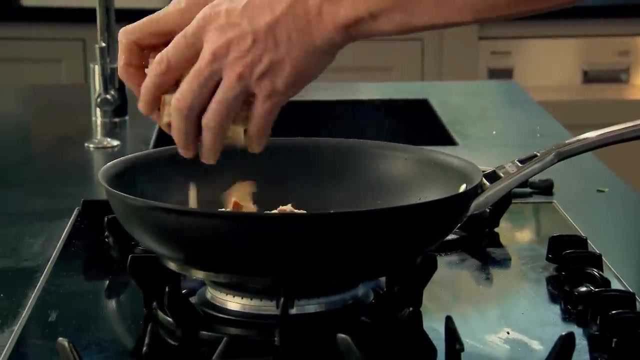 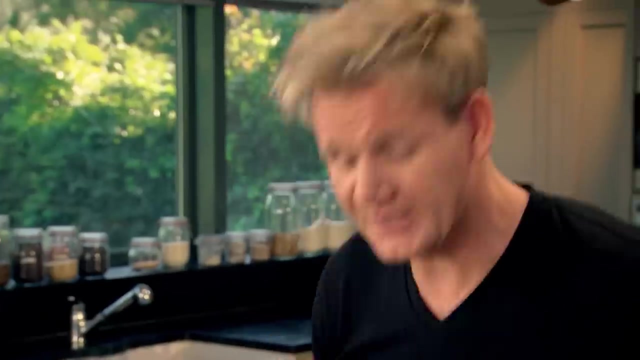 Grab the croutons and squeeze all that excess milk out- Not too hard- I don't want them dry And in- And then just fry them And the milk inside these croutons give it that nice, spongy, creamy, delicious flavor. 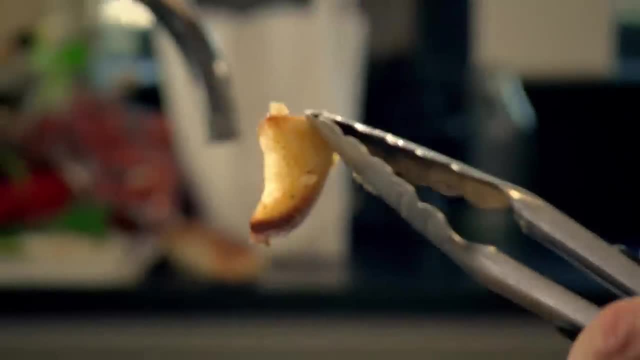 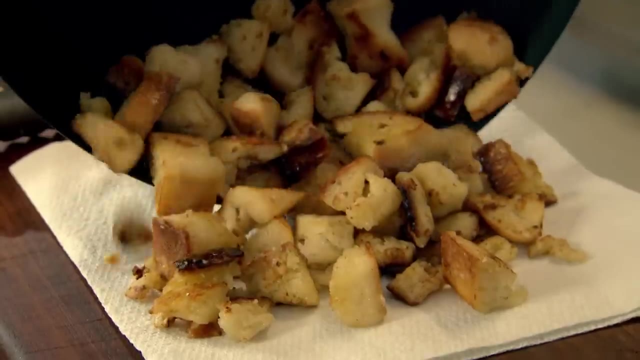 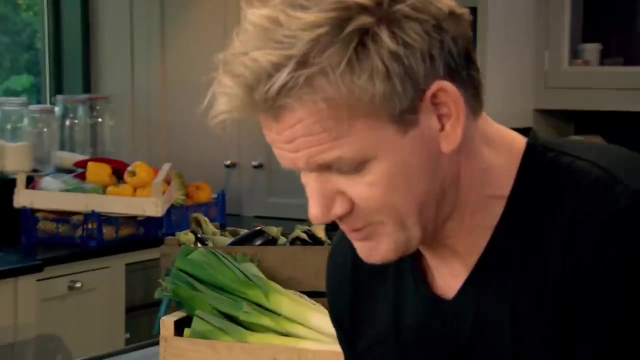 That's the color I want, Nice. Now take them out and lightly drain them. Little bit of kitchen roll onto the board Out, Plate them. Just take this amazing vinaigrette and spread it. Get those croutons. 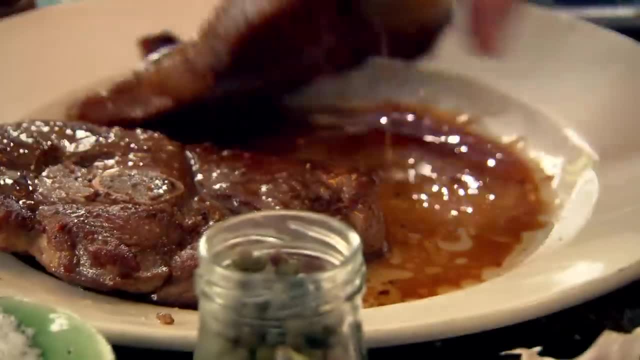 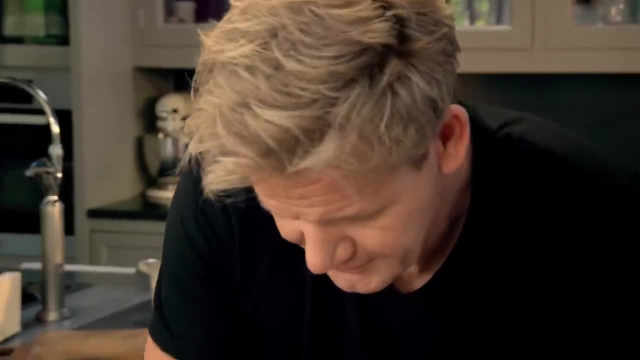 Listen to them Like little boulders hitting the plate. The lamb Sit that on, Next one On The rest of the croutons On. Now use all those little bits And my chef in Paris would kill me right now. 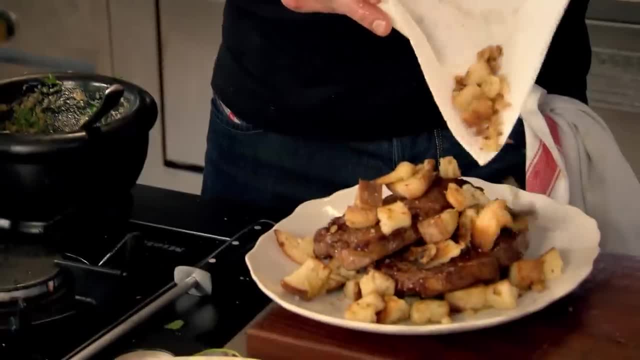 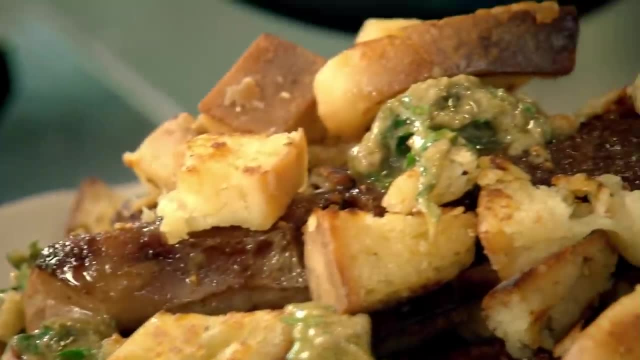 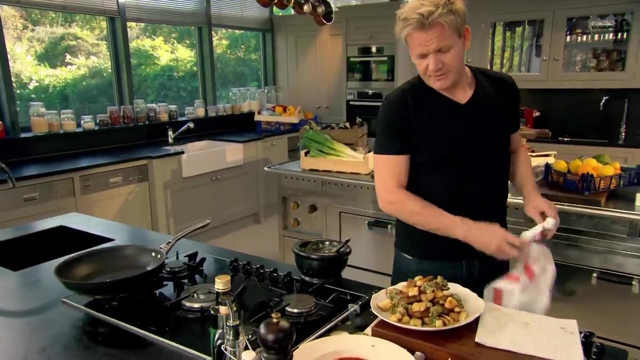 if he saw me using those. They're the ugliest scraps that customers should never see, But they're the best. bits Croutons on And then just drop that sauce on all those little bits of the lamb, And there That is a perfect way of taking a cheap cut. 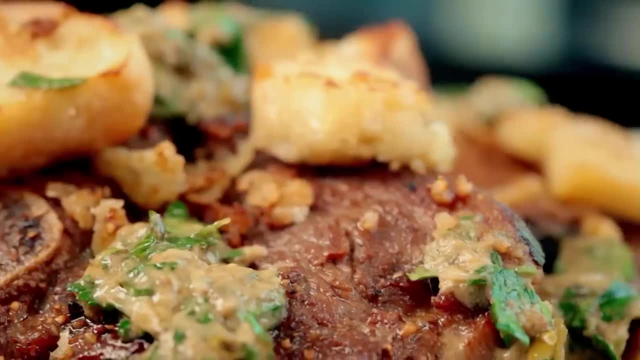 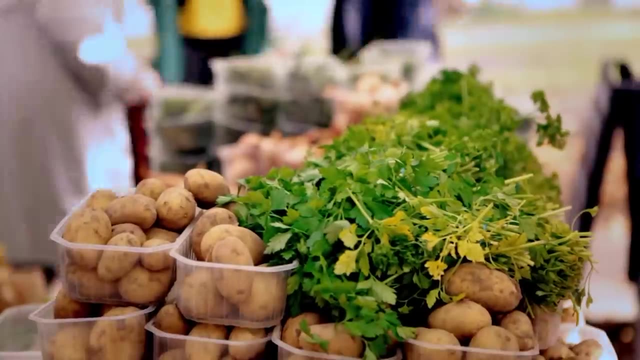 into the Premier League of dishes. Vegetables are such an asset in the kitchen: Healthy, fantastically fresh and incredibly versatile, And pound for pound, They're so much cheaper than fish or meat. Just make sure you give them plenty of attitude. 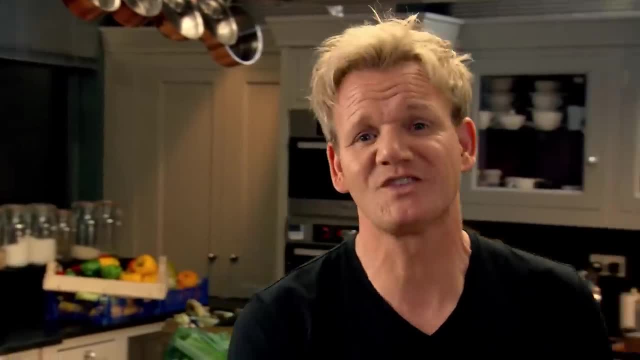 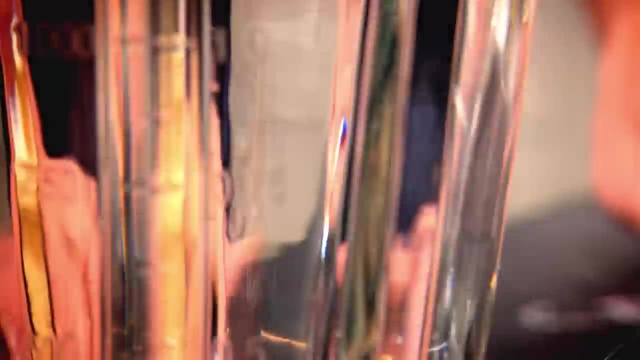 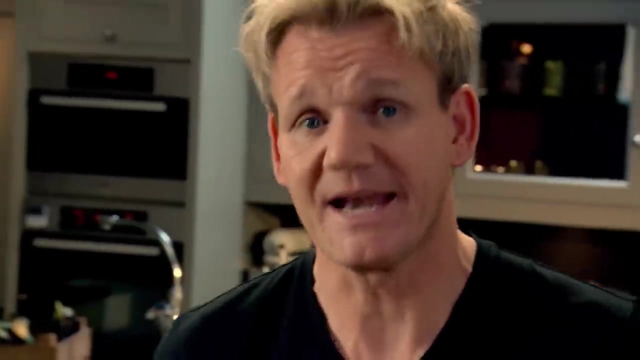 My homemade gnocchi. Making your gnocchi is so simple to do, yet the results are absolutely stunning And it's a great way of using up leftover baked potatoes. You can make gnocchi just with flour and eggs, However. the potato gives it a nice light sort. 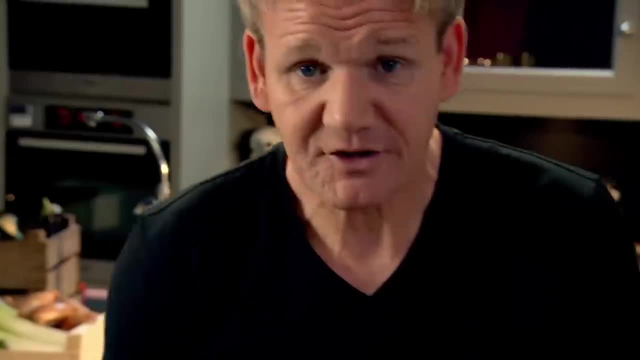 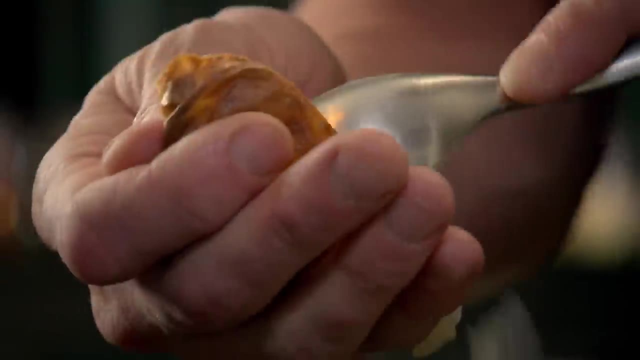 of creamy, fluffy texture. Cut them in half. Take your spoon And scoop the inside of those potatoes. I'm using leftover baked potatoes, But this really works as well with leftover boiled potatoes. Two choices: You can get a fork and sort of mash the potato. 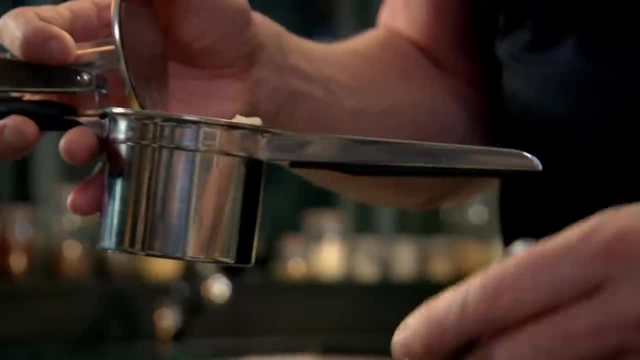 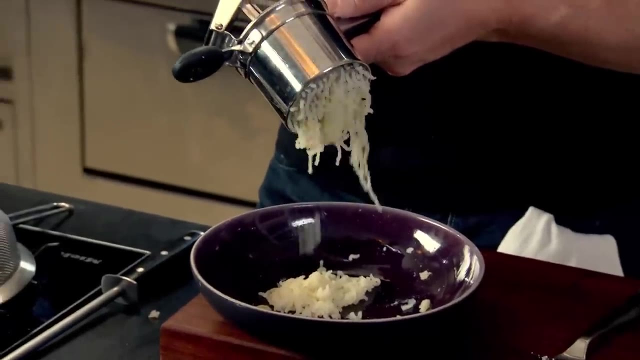 and get it nice and light and fluffy. Or this little gadget- It's called a ricer- I suppose it's a posh word for a potato masher. Just squeeze gently, You can see how nice and light it is- Almost like fluffy little strands of potato. 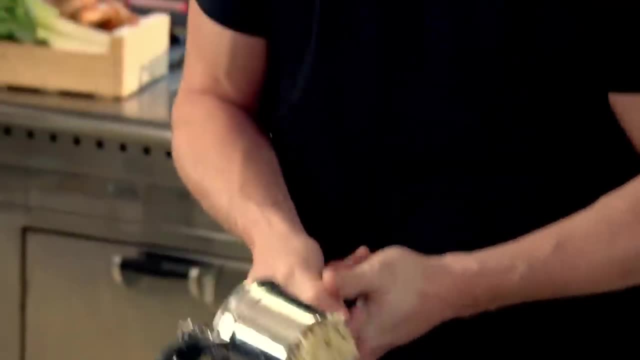 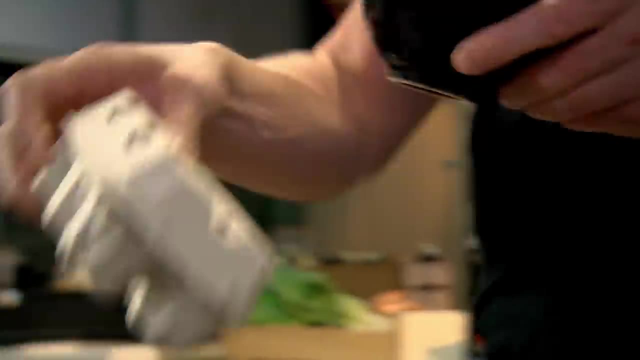 You can do this when the potatoes are hot. It'll go through the ricer so much quicker. Just slice that off. there Now a nice spoon of ricotta in Little touch of salt and pepper. It's really important to season the mixture as we go along. 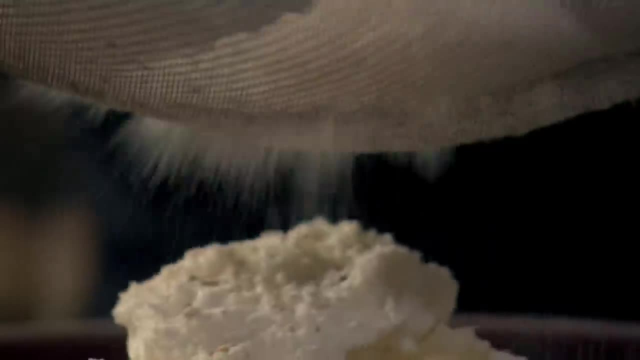 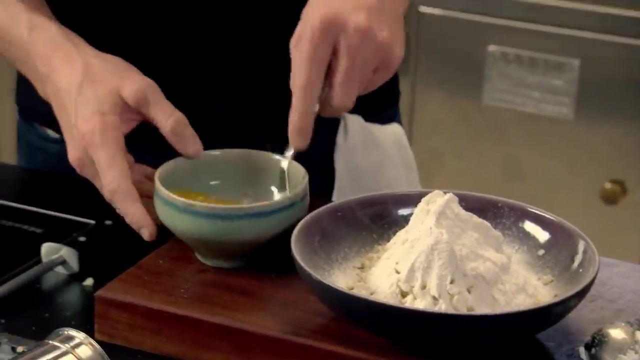 Otherwise the gnocchi becomes really bland Flour over the ricotta Sieve. so there's no lumps. One delicious egg. Give that a little whisk. Now make the gnocchi. You don't want to overdo it. 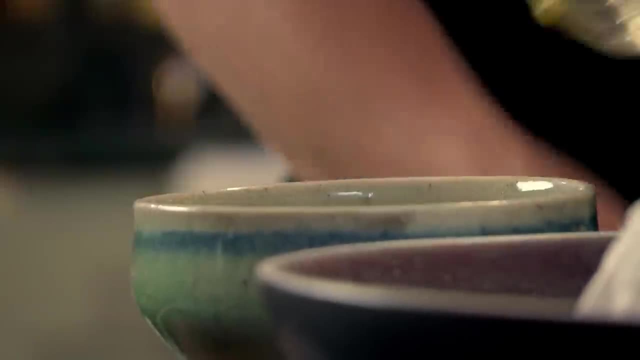 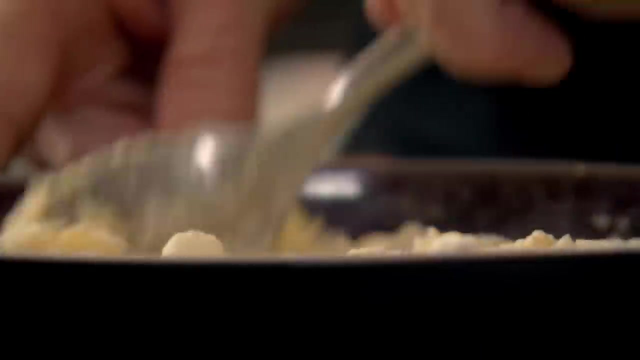 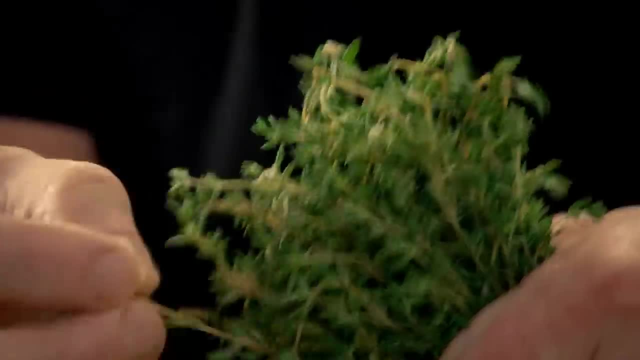 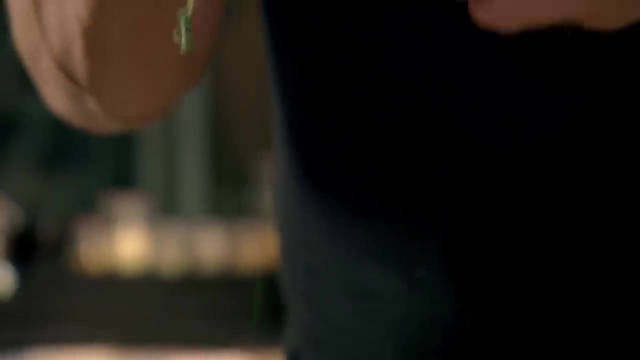 Get some thyme flowers in there, And this thyme is light fragrant And it's just a really nice herb And with the ricotta it tastes brilliant. Just pick the little tips of the thyme flowers, Next flour your hands generously. 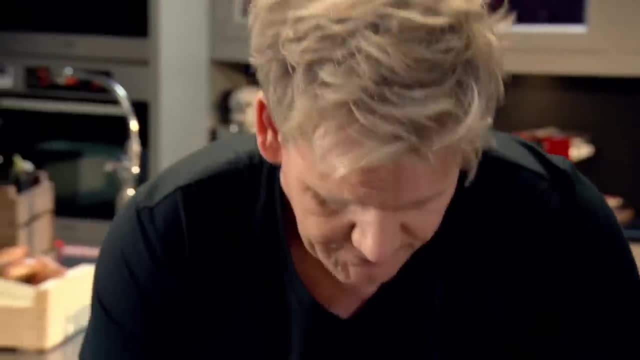 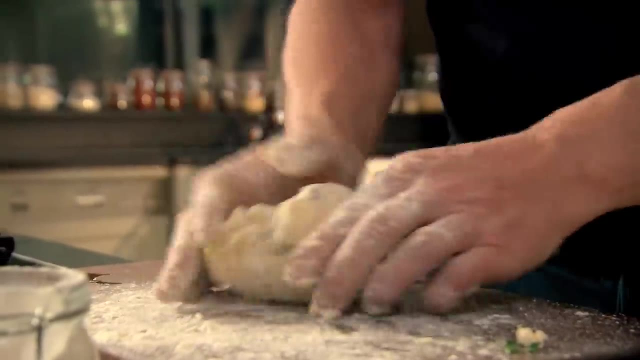 and knead the mixture into a dough, Fold in and push And basically what it's doing is getting nice and smooth. As it starts to get a little bit wet, then just add a little touch of flour. We want something really nice and soft. 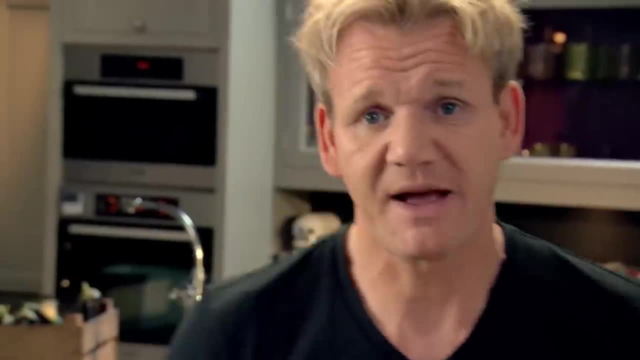 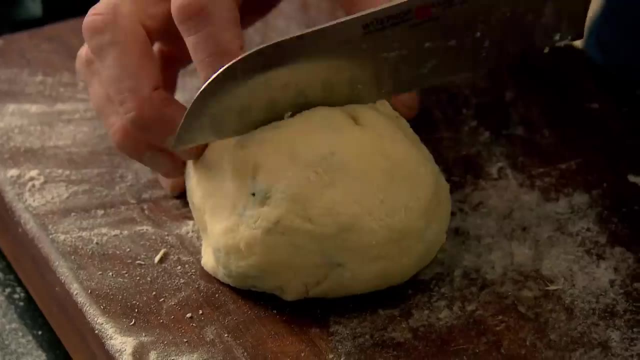 Now, don't overwork it. It stops the gnocchi from expanding when it hits the pan. That's exactly what I want: A nice sort of soft, fragrant ball. Cut the ball in half, Lightly, flour the hands and just roll it gently. 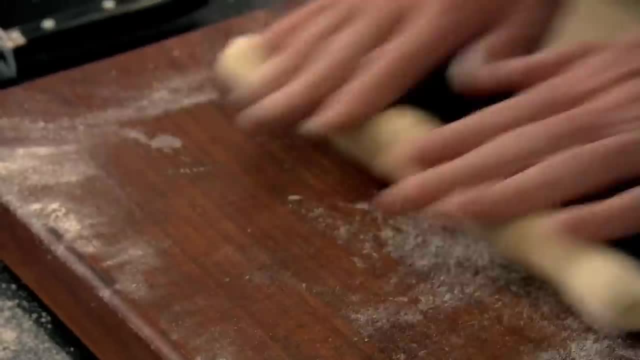 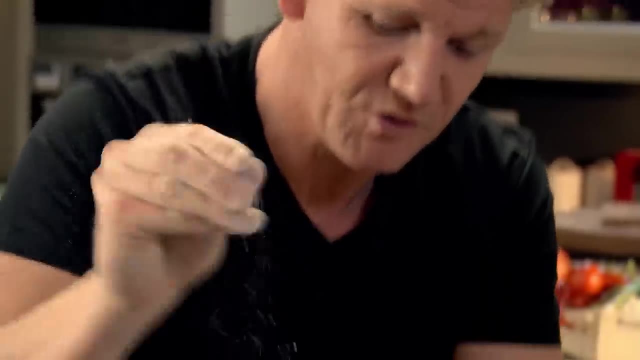 Just think of a big long cigar. The mixture will start getting a little bit sort of wetter, But do not add lots of flour Now. lightly flour the knife so when you slice the gnocchi it doesn't stick. Cut the dough into bite-sized pieces. 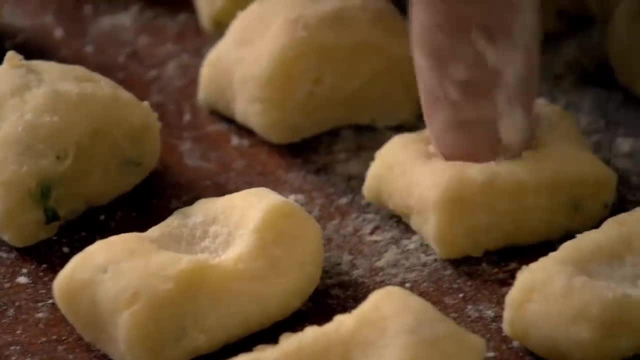 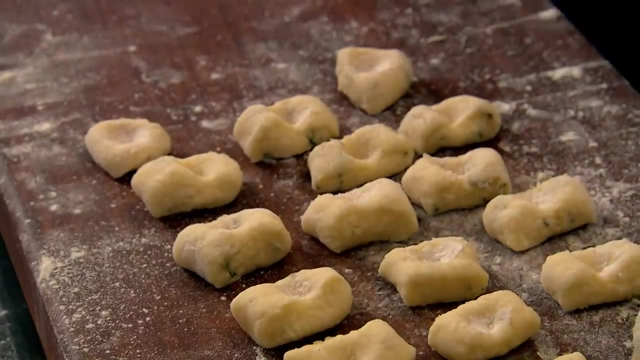 Just take your finger, dip it in the flour and push down. Why I want my gnocchi to look like a pillow And for me, the most important part there is that not one of them are identically the same shape. 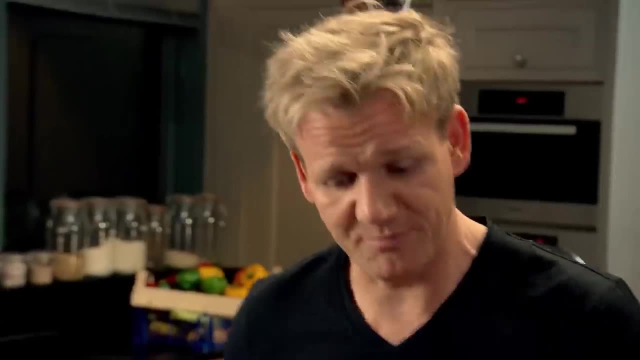 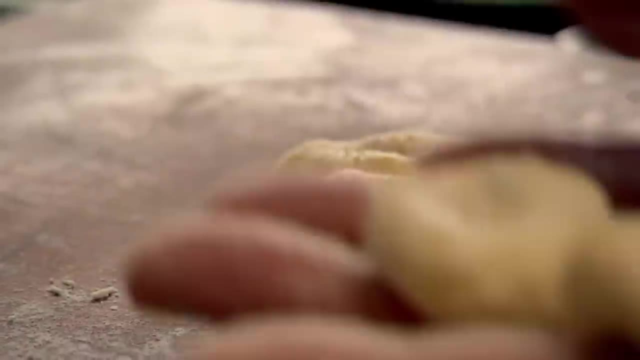 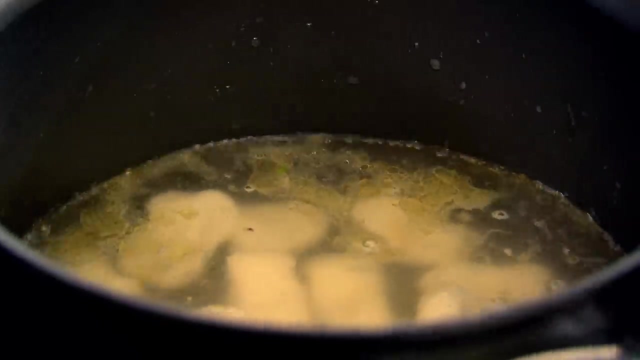 Water on, Bring it up to the boil. A little touch of olive oil in there, Lightly flour your hand, Lift up the gnocchi in to the rolling boiling water, Turn that pan to stop them from sticking at the bottom And let them simmer. 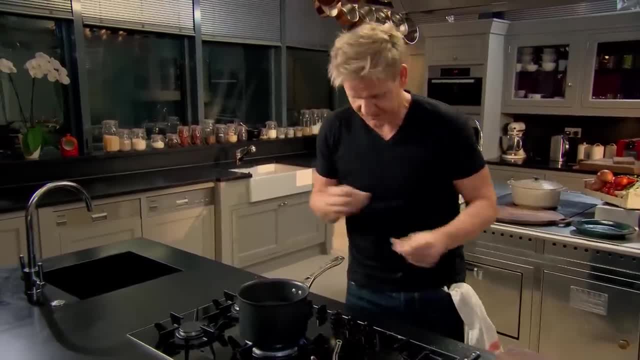 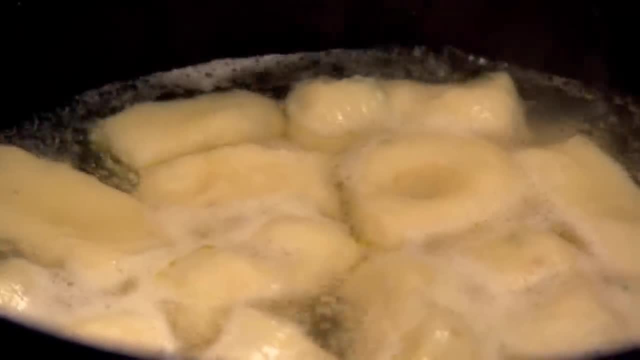 And they start to sort of tell you they're cooked when they start floating. Get a pan on, Get that nice and hot. Now they're just starting to come up to the top And you can continue cooking them like that. I like blanching them in the water. 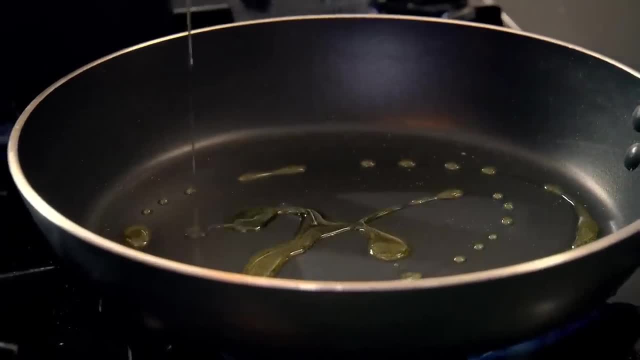 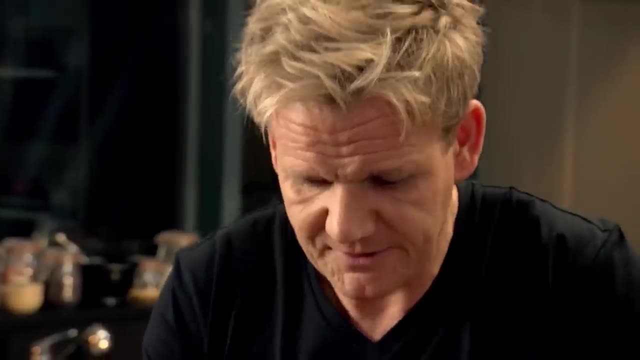 taking them out and then frying them To serve the gnocchi heat off the heat. Olive oil in a frying pan. Gently lift up and look They've doubled in size. Drain it. Get rid of the excess water. 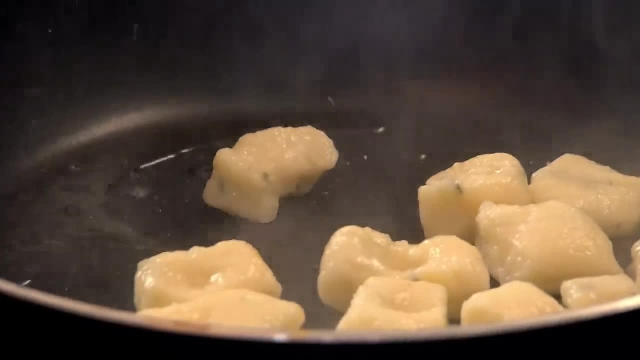 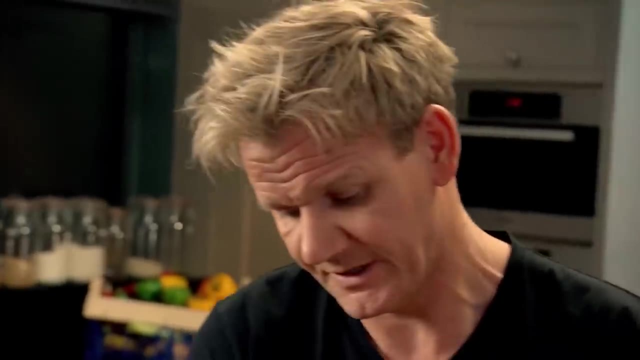 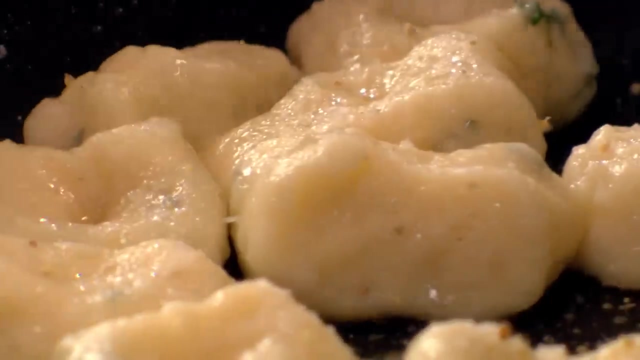 And straight in to the hot pan. This is where they start to take on a completely different texture, a nice crisp, sauteed texture on the outside. Gnocchi loves fresh pepper, So pepper in, And you'll see as I start turning them. 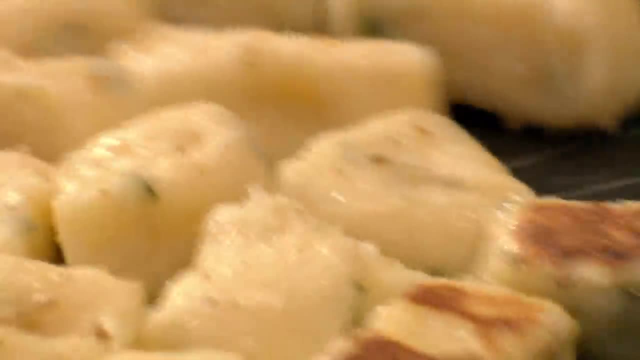 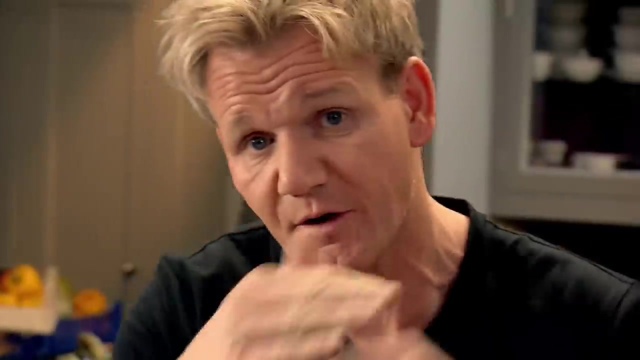 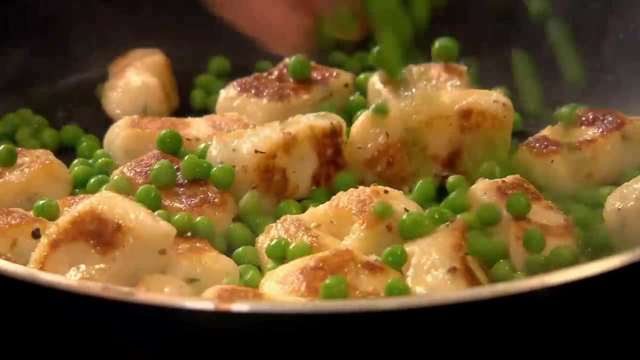 got this really nice little sort of brown color And they're almost popping up now like little parcels. So I want them nice and sauteed both sides, but light and creamy in the center. Fresh garden peas in And the butter gives it that really nice sort. 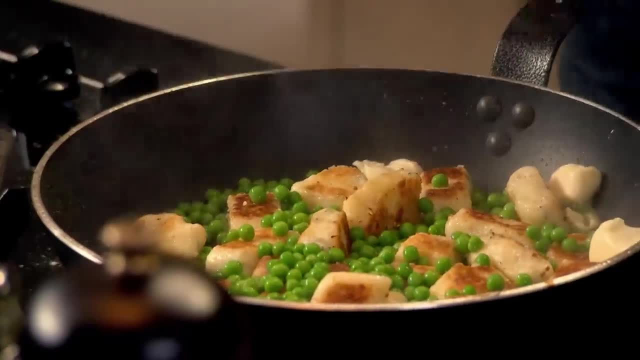 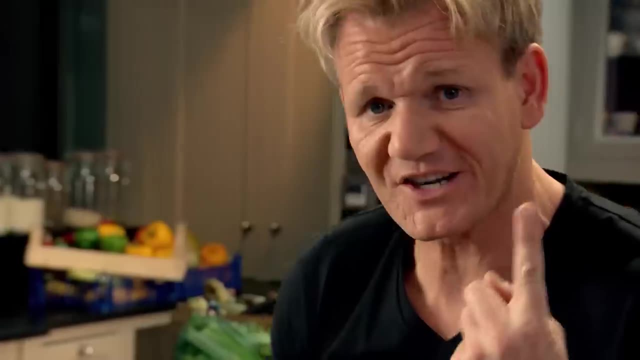 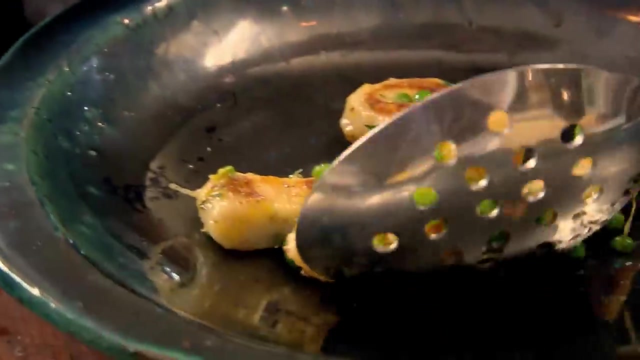 of beurre. noisette flavor on the end, Beautiful. Got a little bit of fresh thyme Over the peas. And then, finally, I want to lift it up: Fresh lemon Zest, the lemon over Serve Smells incredible. 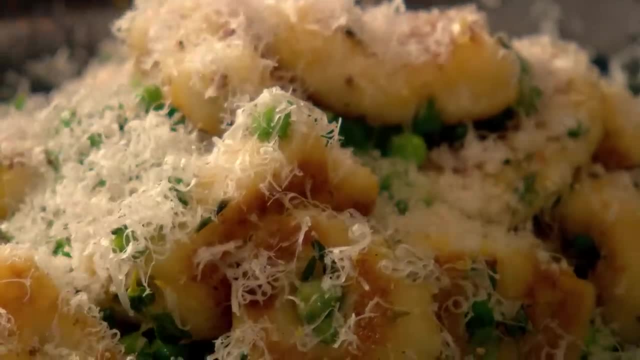 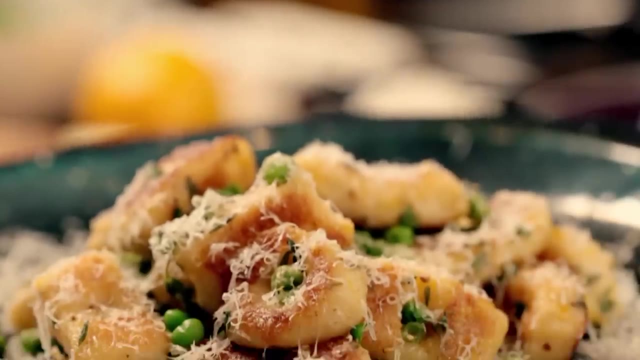 And then finally seal the deal with a touch of grated parmesan cheese. Give your veg some attitude and you'll get amazingly elegant dishes on a budget that are always guaranteed to impress. What more do you want from great cooking Cheap? to make, easy to cook and absolutely stunning. 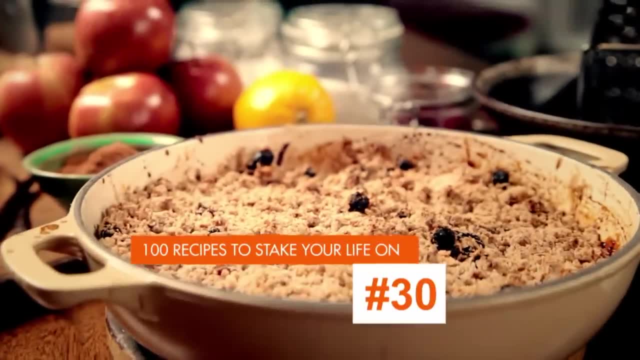 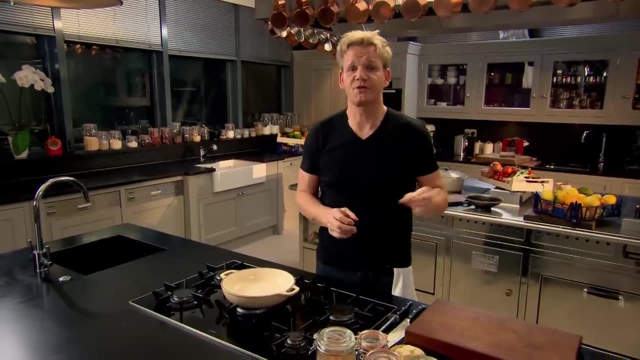 My next recipe is a proper British classic that's super simple to cook and costs next to nothing- a delicious apple crumble. Crumbles are the perfect way to use fruit when it's in season. There's lots of it about. It's nice and cheap, but most importantly, the fruit's. 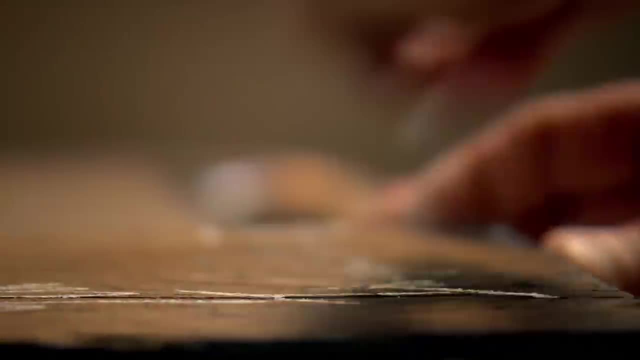 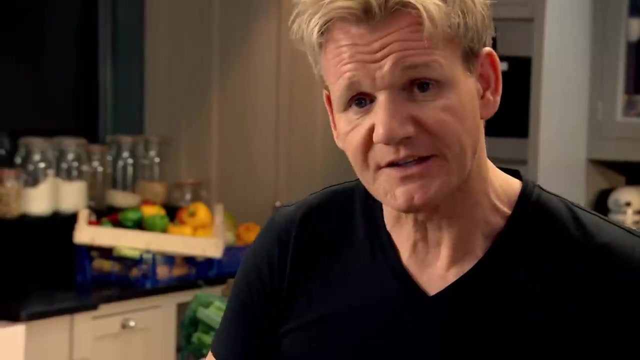 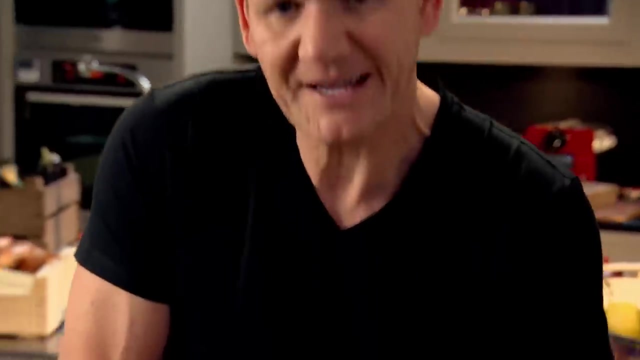 at its absolute best. First off, I'm going to make a really nice light caramel Pan on nice and low Grate two apples, And this helps to almost sort of pure the apple so much quicker And there's a lot of flavor in the skin. 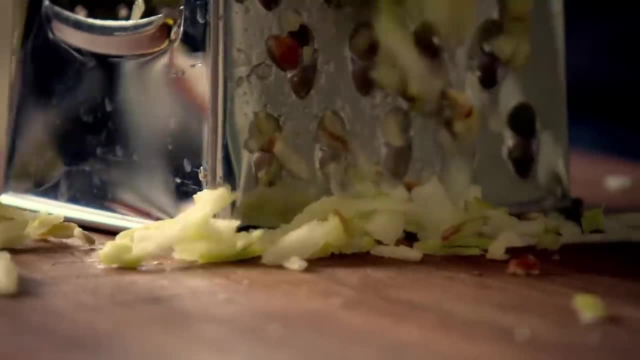 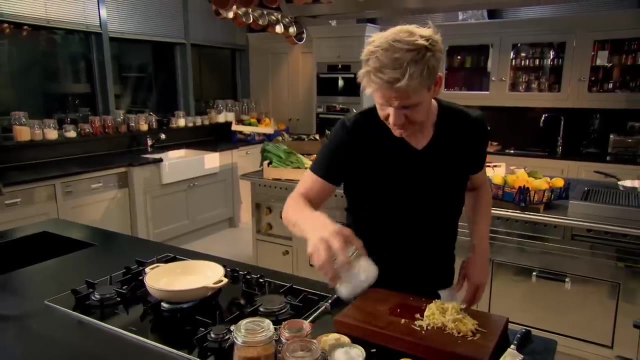 so don't worry about peeling the fruit, Whether it's pears, plums, peaches, the flavor's in the skin. Nice To start the caramel: a couple of tablespoons of sugar. The sugar helps to get rid of the tartness in the apple. 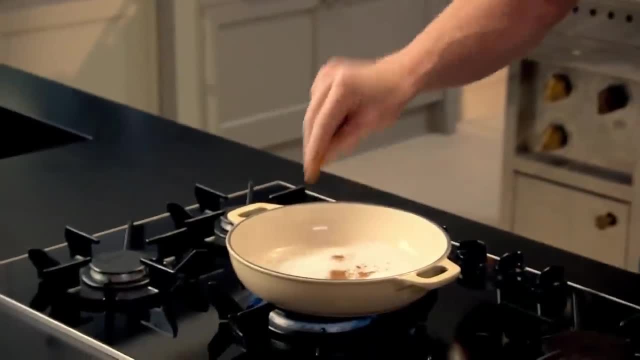 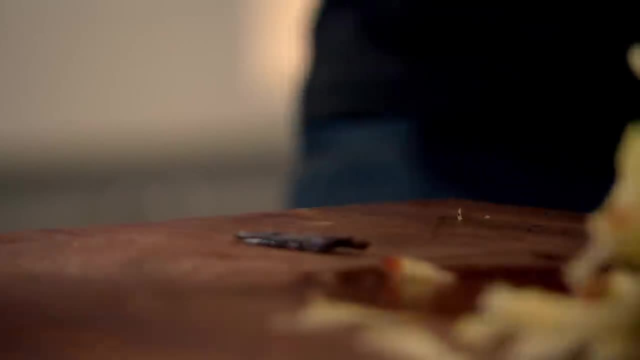 A touch of cinnamon, That starts to make it a little spicy. Open up your vanilla. Just scrape out all those seeds Now. this just makes it light and fragrant. All those seeds in to the sugar When making caramel. be patient and always swirl. 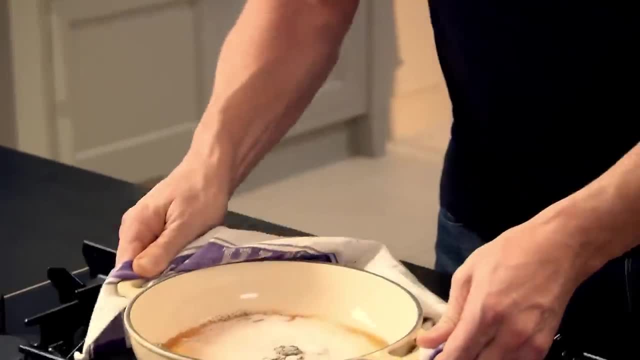 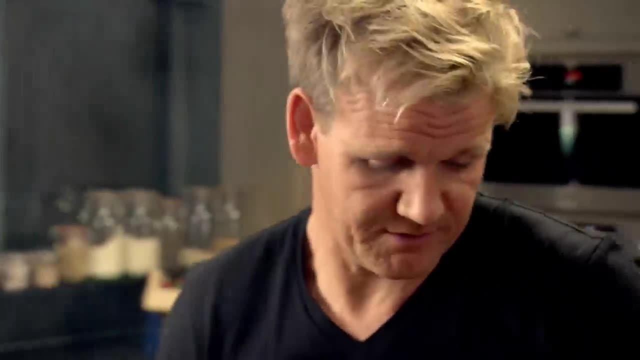 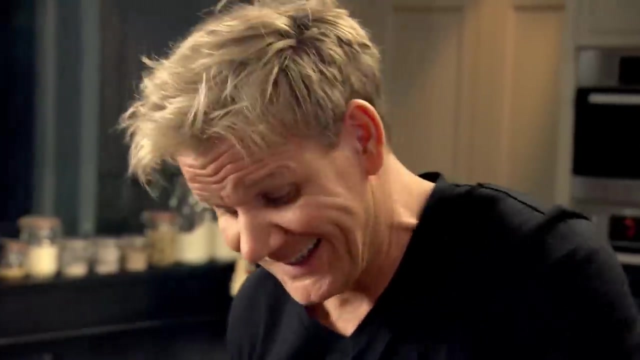 the dish instead of stirring it. When the sugar goes brown, add the apple. That starts to sort of cool down the caramel, but it gives it a really nice sort of caramelized puree. Apple's almost disintegrating Smells incredible. 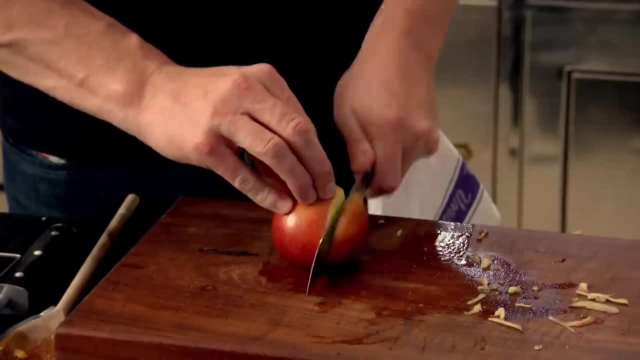 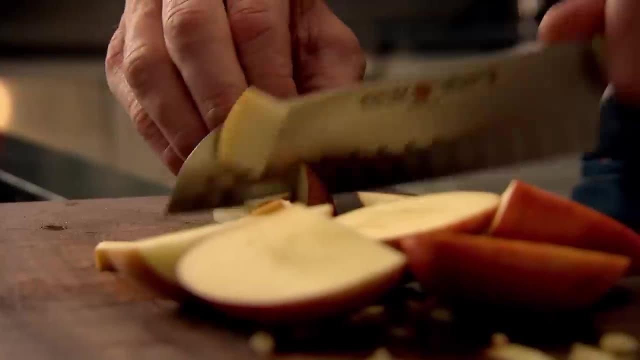 Turn the gas down, Slice up two apples. It's a crumble that's got no frills, Straightforward, No faffing around, No peeling of the skin. I want them to sort of stand out from the caramel Apples in. 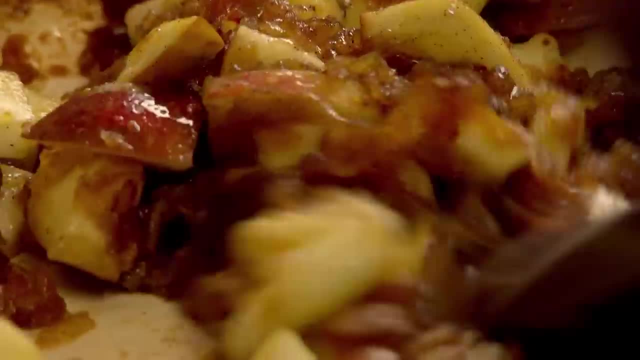 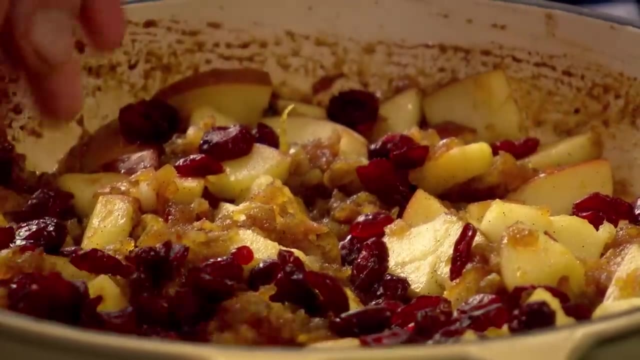 Now those nice thick chunks of apple are sort of almost bedding itself into the puree. Dried cranberries gives it that nice sort of shock in the texture. Sweet and chewy. I want it to sort of taste zesty, Spicy. 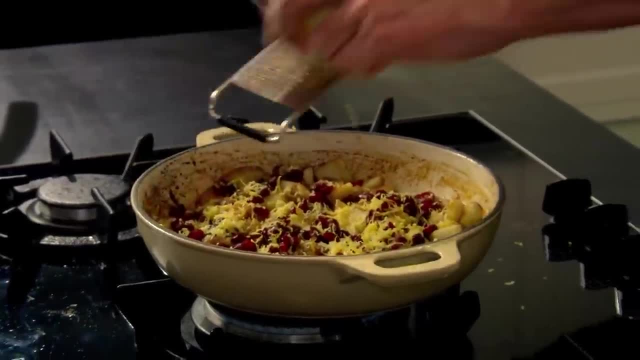 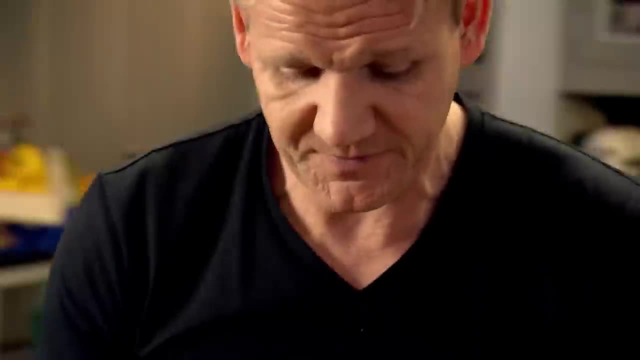 So sit the lemon zest on top of your apples and cranberry Fresh lemon juice over And that just gives that extra acidic kick. Takes the cranberries, the apples, the caramel and the cinnamon to another level. Turn the gas off. 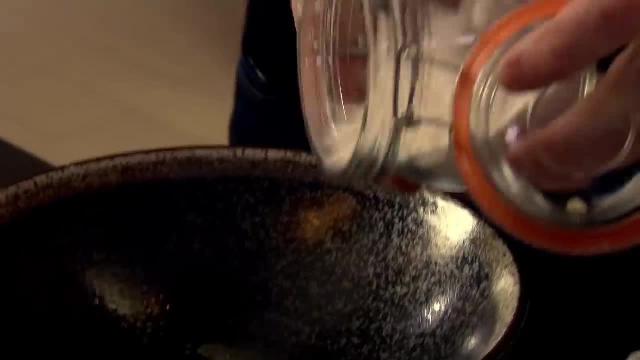 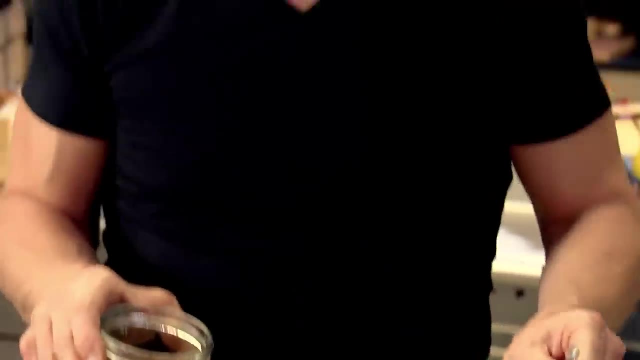 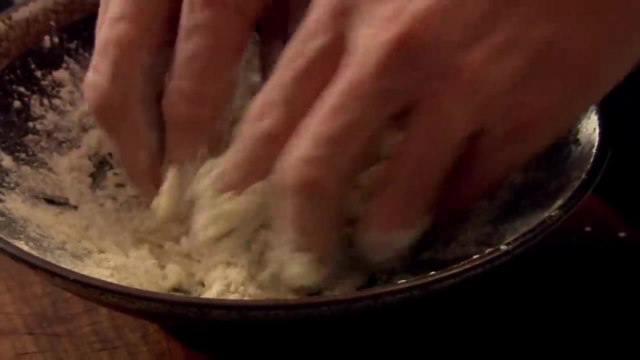 Just let that sit And let's concentrate on the crumble Flour in A couple of tablespoons of demerara sugar. Sugar helps to get the topping nice and crispy. Butter in Give that a nice little sort of rub. What we're looking for is like a breadcrumb mixture. 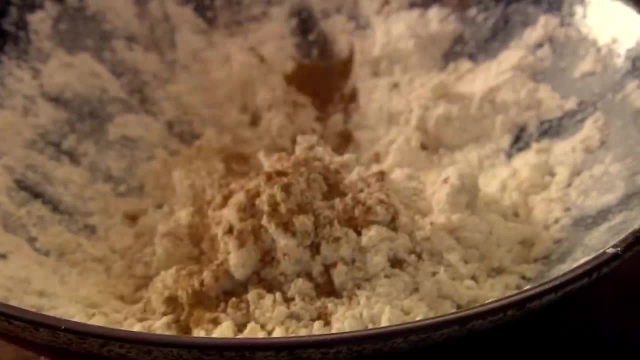 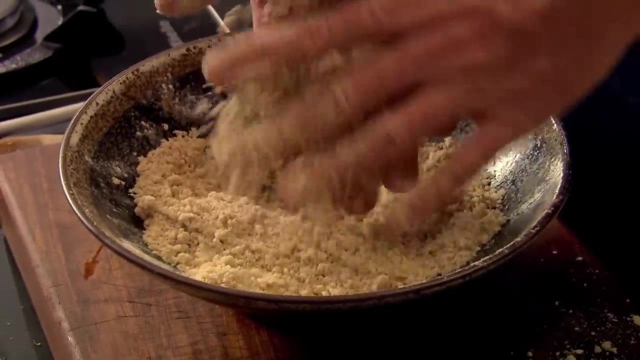 Lightly season it with a touch of cinnamon And the demerara sugar sort of helps to get a nice fine crumble mix And it stops the butter from sort of melting in that flour. So that's the basic crumble mix.